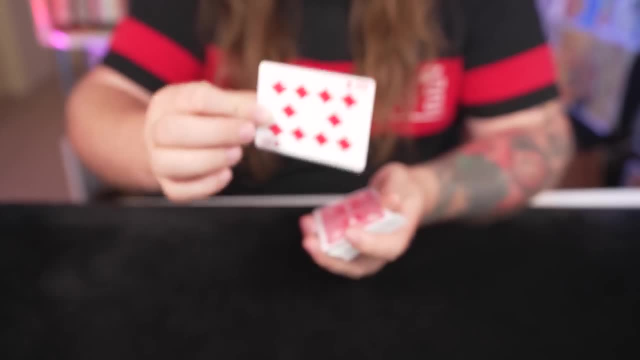 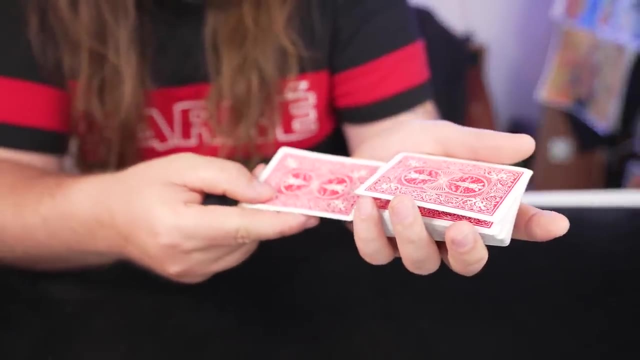 just looks like a regular deck, so don't overthink it. Now take the card back from them, remind them of the card and then you're going to seemingly place it in the middle. but what's going to happen is I'm going to use this card to push forward a few cards from the middle and then I'm going to 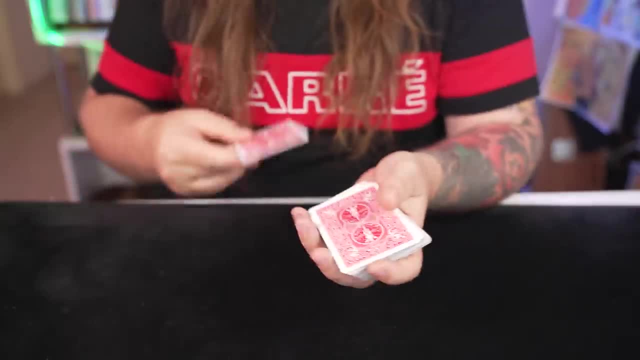 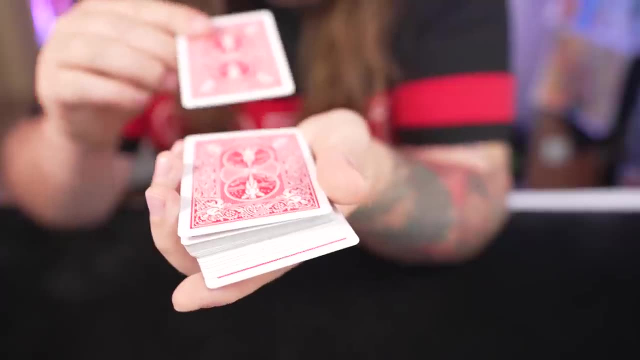 place it directly second, from the top. Now, the reason why I do this, the reason why I push a few cards from the middle first, is it creates this illusion that it's really going in the middle watch. as I place it here, it really looks like it's going somewhere in the center of the deck. 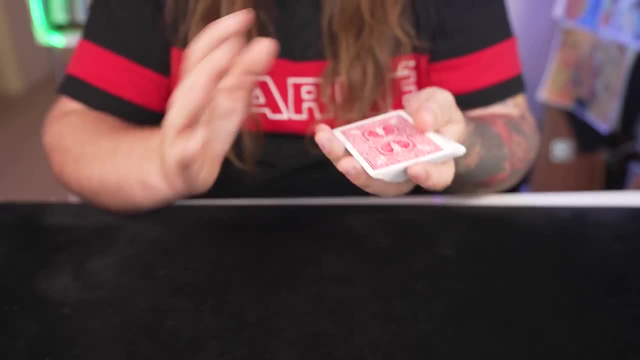 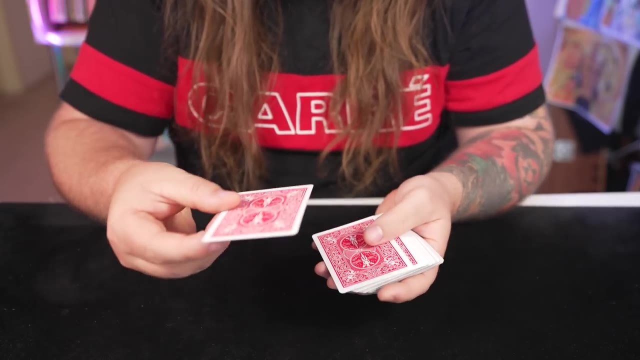 because of this right, and once I square everything together, it just looks so good. Now, from here, it's second from the top, and all you're going to do is you're just going to pick up the top most card and say, bam, is that your card? which they'll say no, but while you're showing them this, you do the. 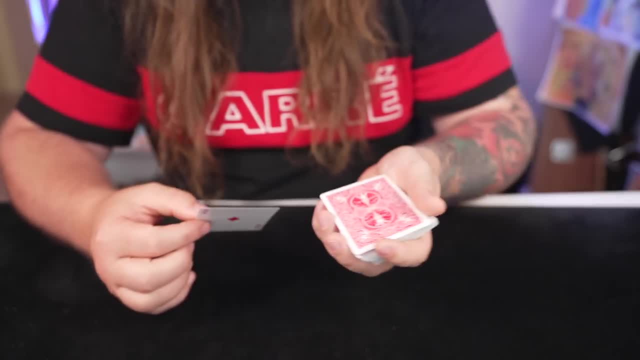 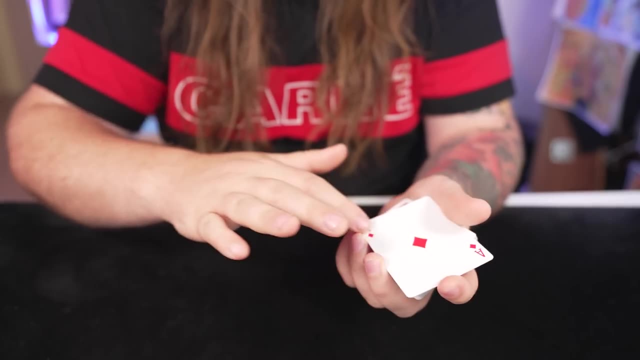 same thing again. you push this across. you put your pinky underneath, holding it separate from the deck, place that card on top of their card and then you're going to pick up both cards from corner to corner. we're talking lengthwise, baby. pick them up from corner to corner like this and the motion. 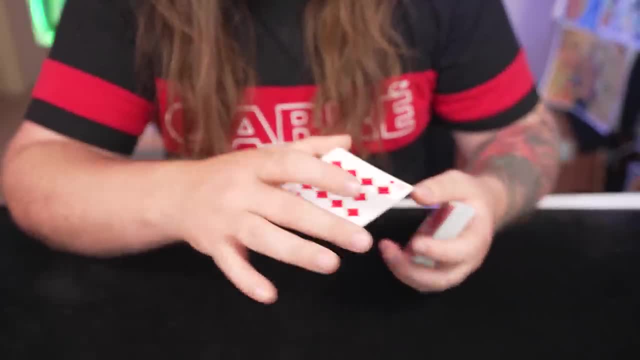 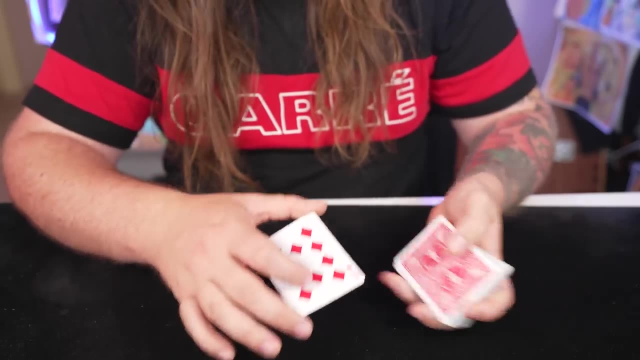 literally is this: you're just going to turn the cards like that, but you're going to do it under a wave, so you're going to shake your hand like this and just at some point you're just going to flip it like that and that's it. and if you really get the timing on this down, it really does just. 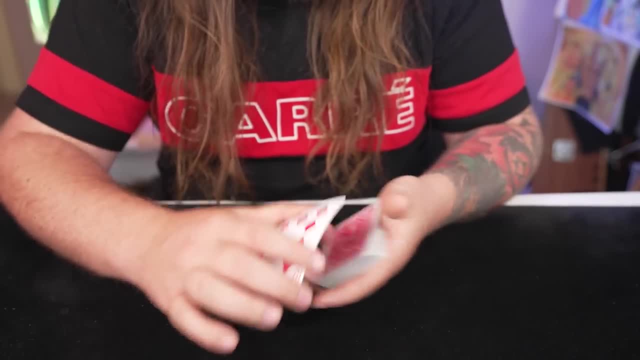 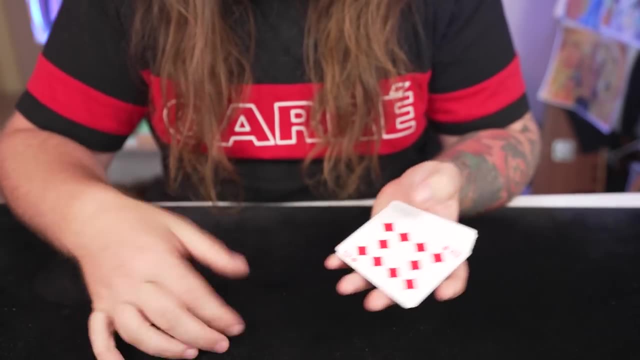 look like that card changes visibly from there. you're going to take this card once you've changed it right. so you pick it up, do your little wave and then you're just going to drop them both on top of the deck and you end clean. you can then take the card off, show the front, the back they. 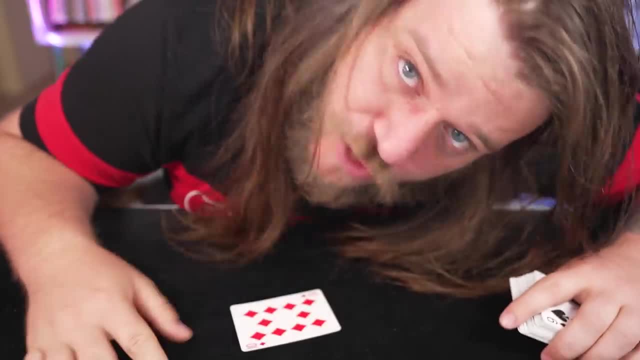 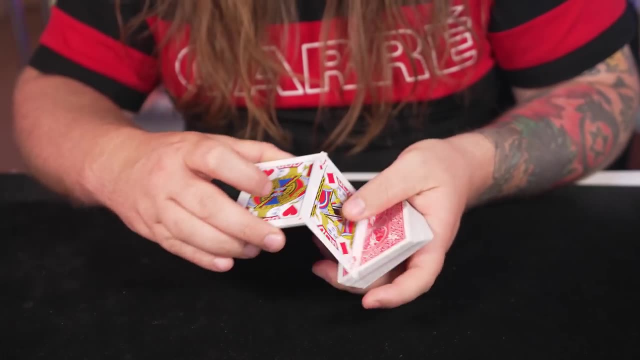 can check it out. it's a bona fide miracle and it's literally super easy. pretty sick man, but no time are wasted. we're moving on to trick number two. baby, all right, here it is trick number two. get in nice and close for this we've got the jack. 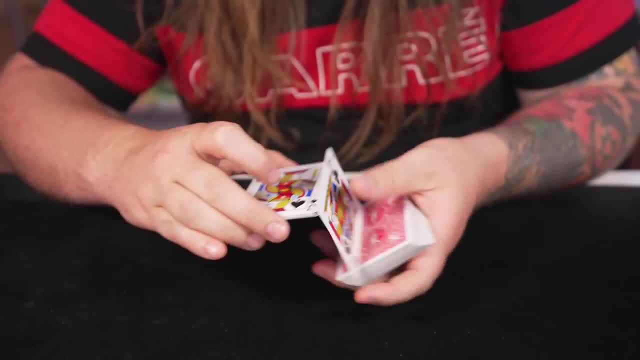 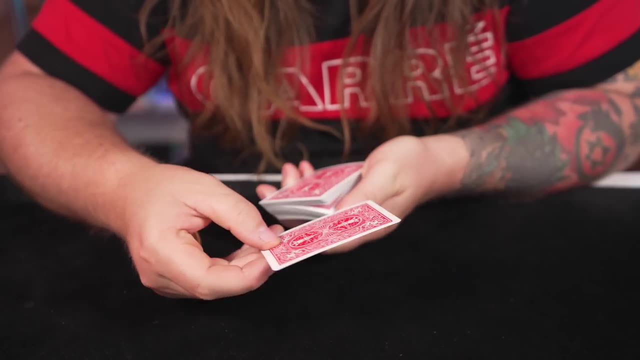 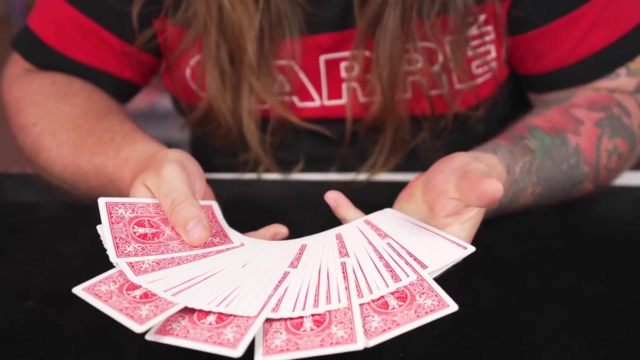 of doymans, the jack of freaking hearts, the jack of l clubs and, last but not least, the jack of spades. and those cards are going to be placed into the deck in separate areas. look at that man. all of them in the center of the deck, in different areas, and when i push them flush i turn the deck. 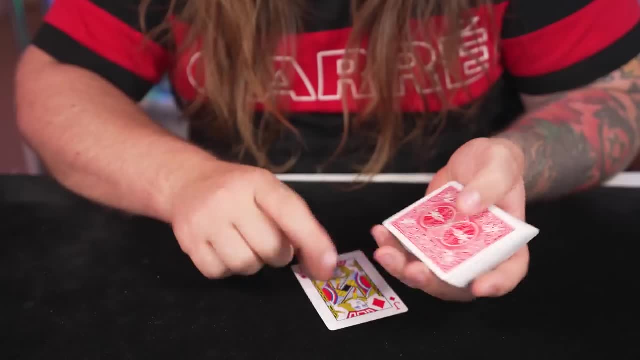 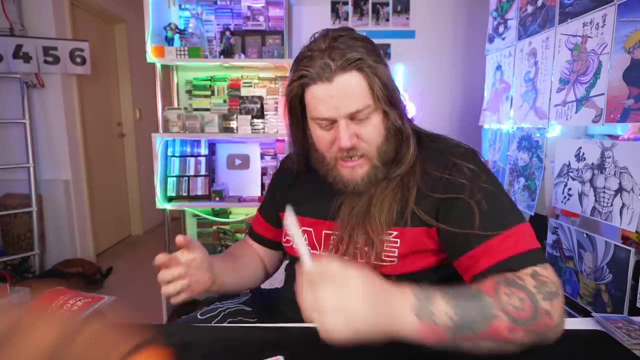 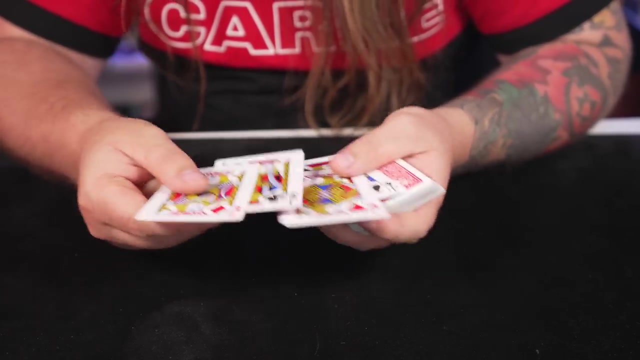 like this. i snap the fingers. and you guessed it, baby. one, two, three, four jacks. they're back now. isn't that a bloody sick trick? all right, beanie's on, i feel better. all right. so for this trick, you're going to need to have four jacks on the top of the deck, and the way that the routine starts is: you're just going to. 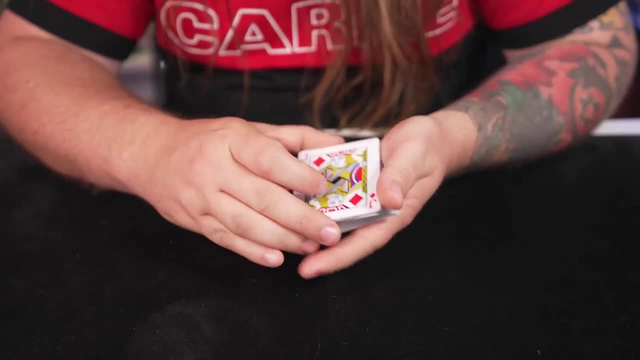 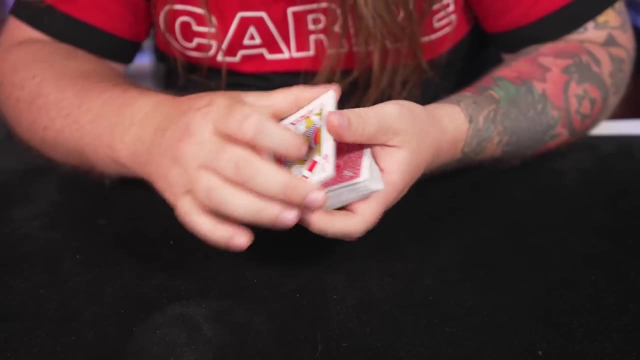 count them off, sort of introduce them one by one. you're going to pick up the cards looking like this: but i actually have four jacks and then four random cards, all held together in a nice little block. yeah, so i'm going to pick up the cards and i'm going to pick up the cards and i'm going to 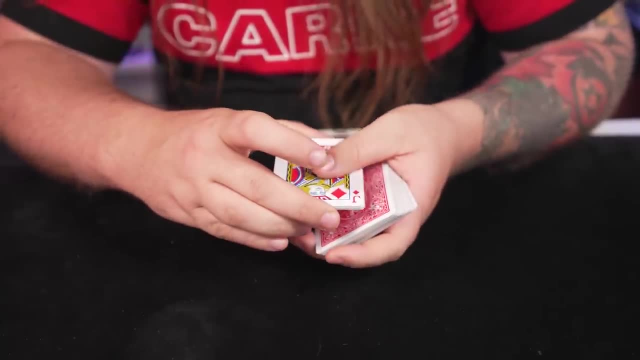 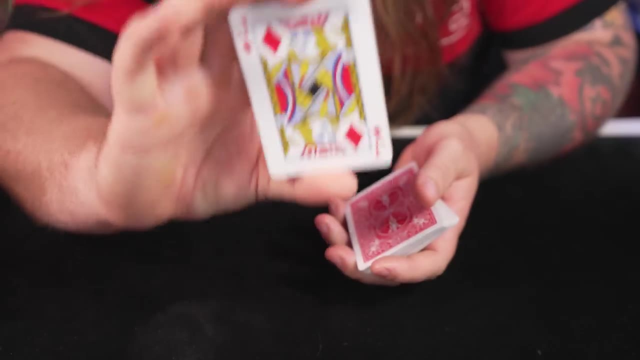 just grab the packet like this and using this hand i'm going to use my thumb to drag one about halfway off- i lever it like this and then i add it to the bottom of this pile so that'll hide the the random cards there. but i do that as i introduce them one by one. so this is the jack of diamonds. 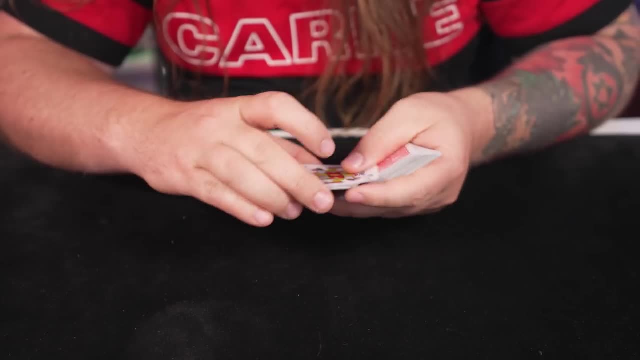 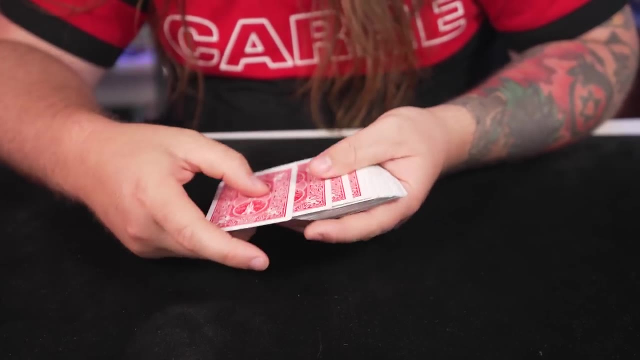 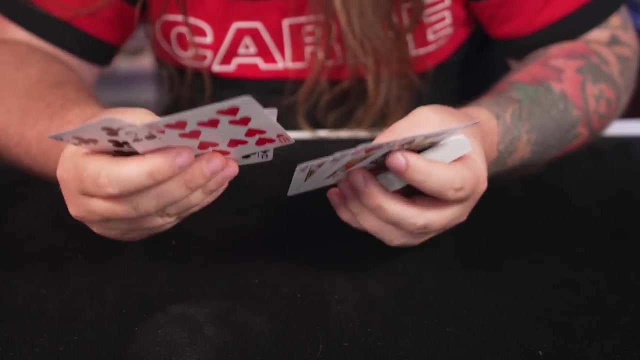 jack of clubs, jack of hearts and, last but not least, the jack of spades. then i can throw the entire packet straight on top of the deck. and now what's happened is i've managed to successfully switch the order of the cards so that now the jacks are underneath four random cards. so once 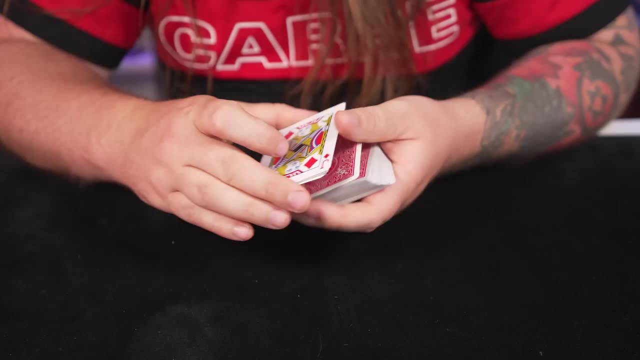 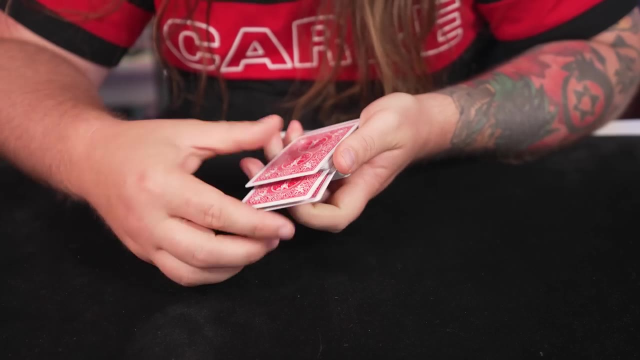 again. i introduce each one, one at a time. okay, i'm just going to speed run through this real quick and then, once they're all introduced, i slap them down and i put the indifferent cards into the center of the deck in different areas. now, what's cool about this trick is that you can spread the 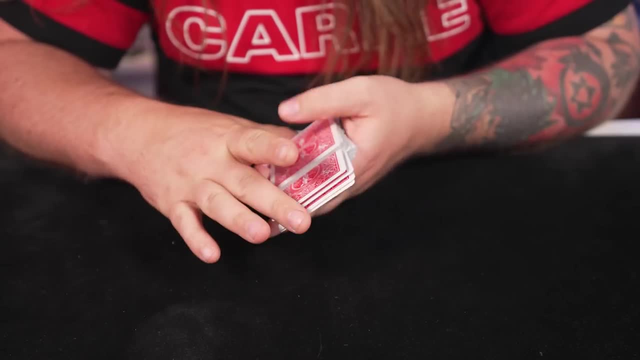 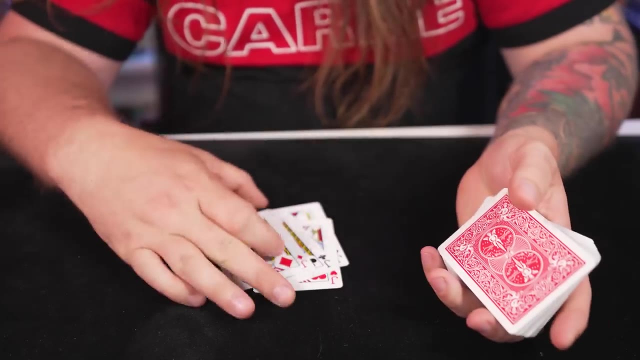 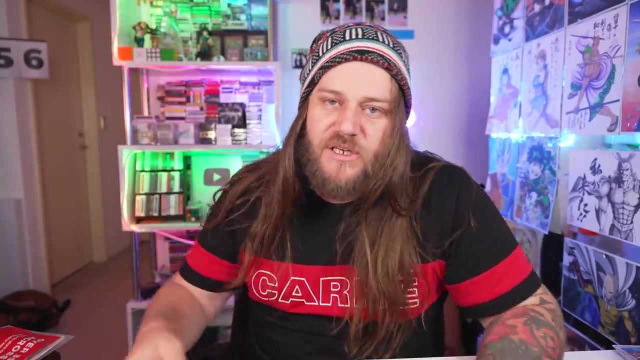 cards out, to show the cards all in different areas, and then when you push them, flush and snap the cards, they all arrive back on the top. it is an instantaneous miracle, and it looks so sick. it's also one of those tricks that's only limited by your performance, so you can like tell a story or 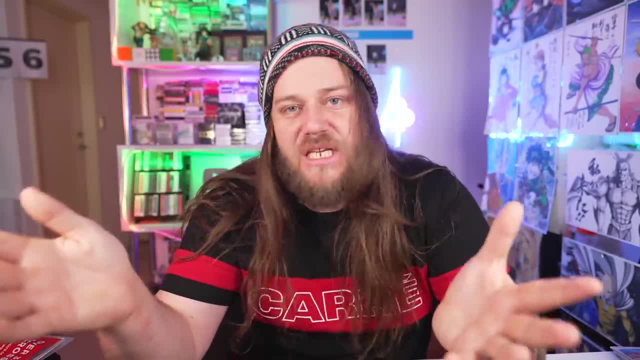 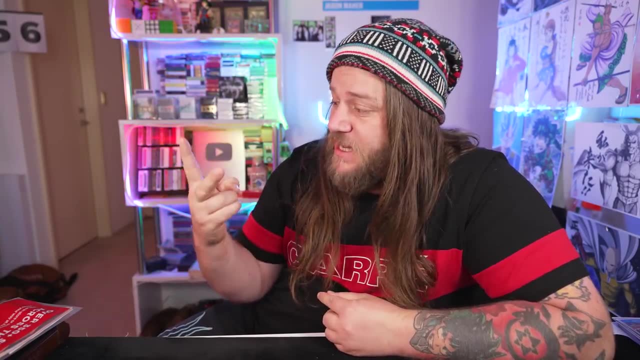 you can make it look like you're a card gambling super genius or something. you can do all kinds of cool stuff with it. all right, so so far we've managed to teach you a super visual, color changing card. we've also managed to teach you a really awesome four card control. i think it only makes 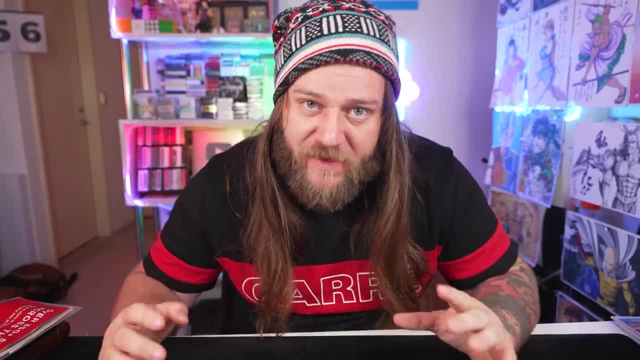 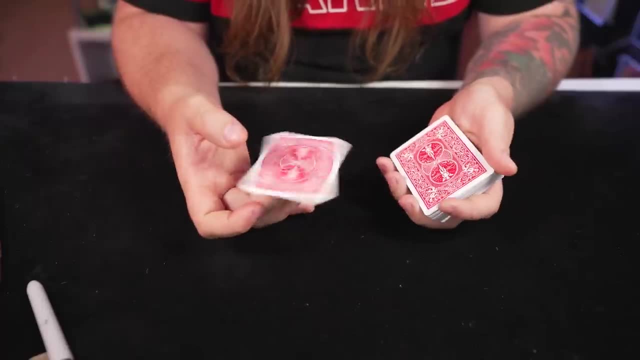 sense that the last trick is a vanish, and not just any vanish, but the last trick is a vanish, something that i use all the time, but it is so easy to learn, trust me, you'll be doing it in no time. all right, here it is a super easy vanish. i'm going to take a card. i'm going to leave it. 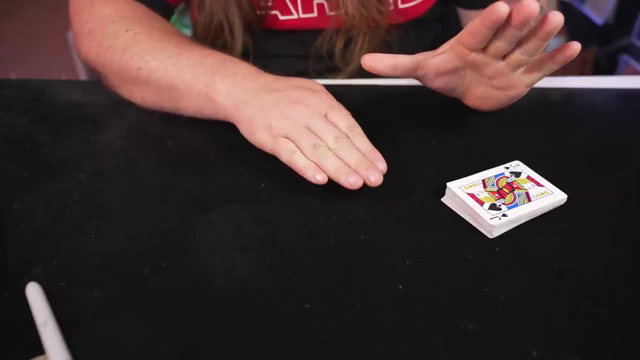 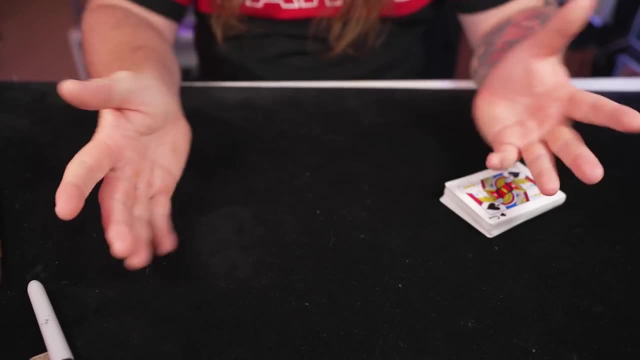 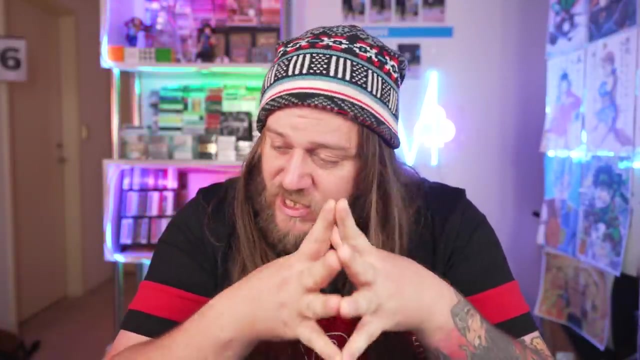 underneath my hand and when i snap the fingers, the card disappears. oh, i know you don't believe me, but look, it really is gone. there's absolutely nothing to see. it's gone. and that right there is the rubber dub finish. now it looks like it'd be hard to learn, but it's actually diabolically. 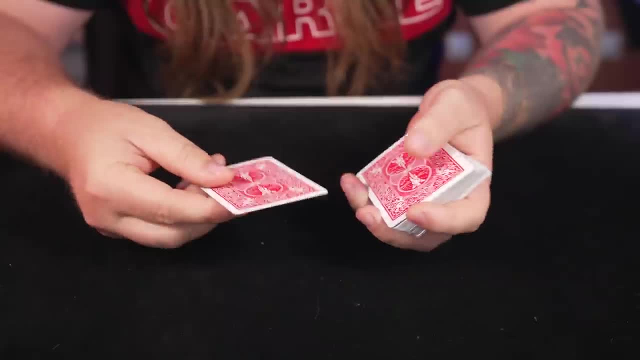 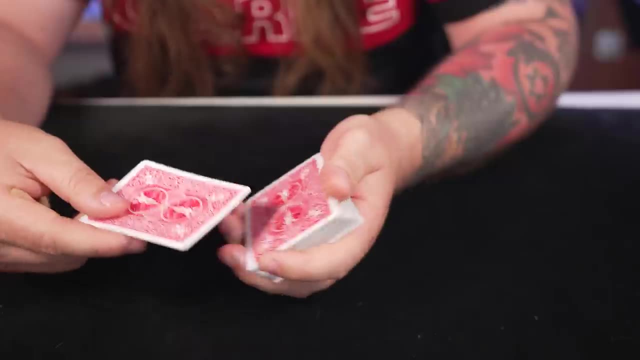 easy to learn. all right, to execute this sweet maneuver, hoover, you're going to take a card and you're going to hold the deck like this right- this is a pretty standard way to hold the deck- and you're just going to insert the card the middle of the card, right up against the finger. 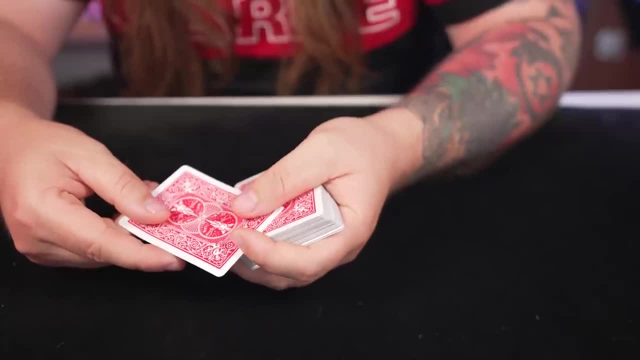 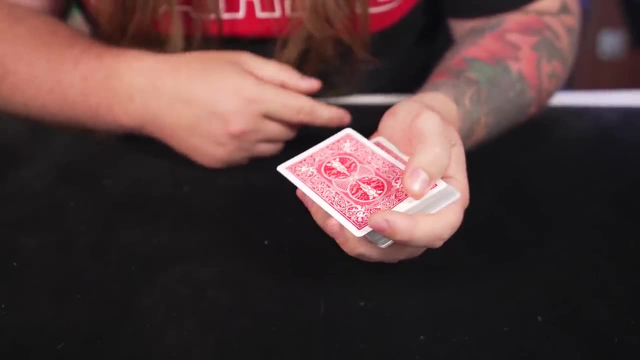 at the very front. your thumb is going to reach over and grab the corner like this. you're holding it like this. this is going to be a lever point, so your thumb, when it pulls back, is going to use this as a guide to build it to align perfectly with the rest of the deck right. so it'll look like this: 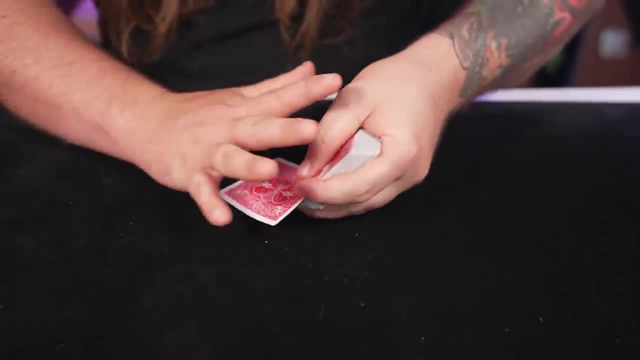 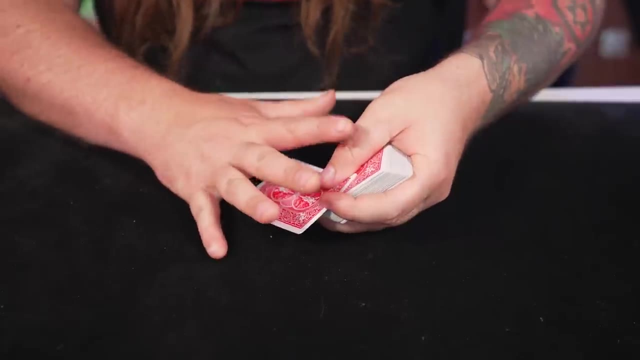 okay. so now we're going to take a card and we're going to hold the deck like this, and we're going to hold the deck like this. now you're doing that under the cover of your hand, you're going to pull this in as you cover it up, and all that really happens here is that the timing is very. 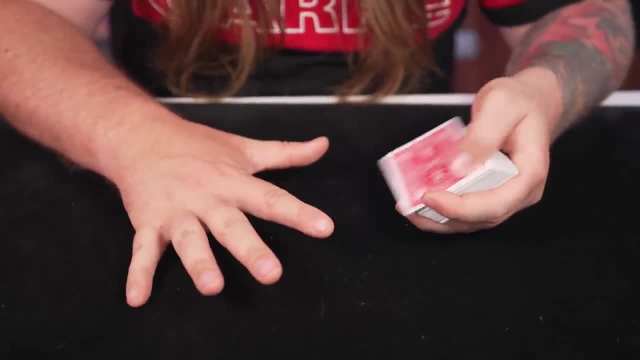 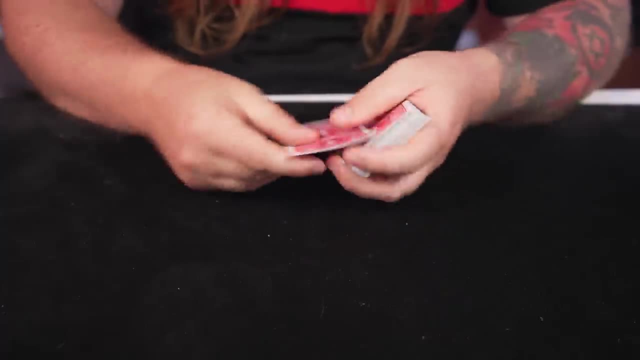 important. so i always come in, fingers spread and then, right as i'm going to pull this card in, i close the fingers, supposedly hiding the card. so i like come over and then i like do this, so it's like i'm covering the card and in a single motion. this is going to be exaggerated, but in a single 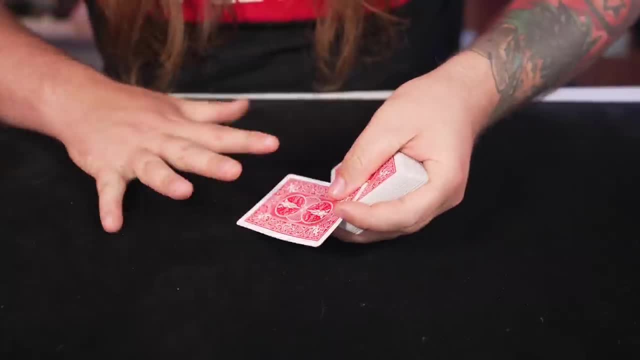 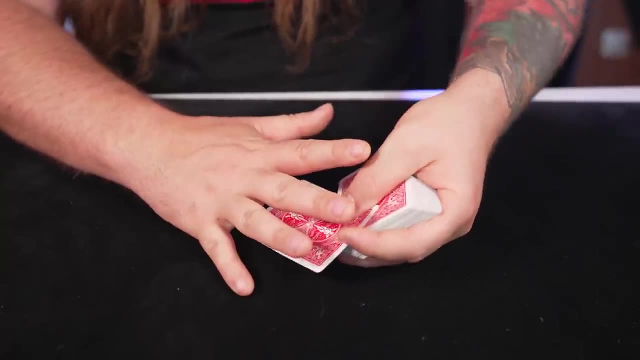 motion. it'll be kind of like that: now, at this point here, you can still see the card getting there, but the trick to hiding that is that i'm going to turn this hand like this. i'm going to turn the hand as i pull it in, and now you can't see it as well. so what happens is i'm going to 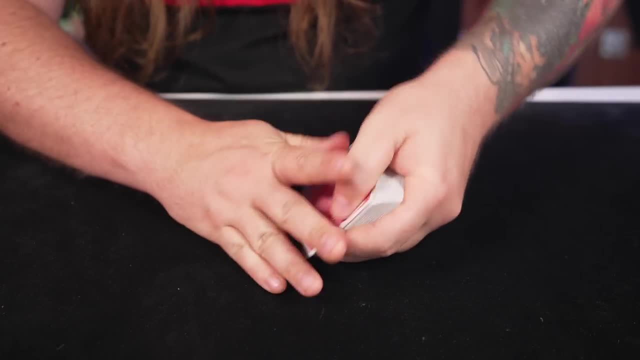 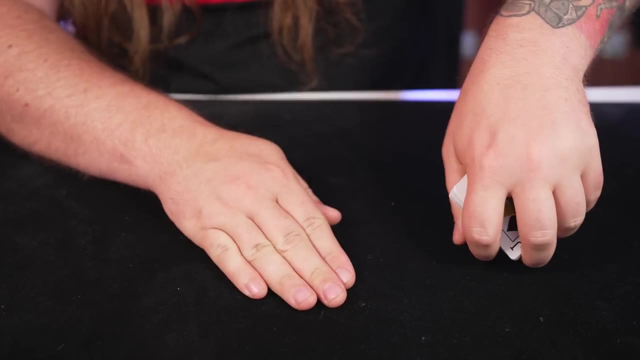 put it here. i turn it as, i cover it and look, i can even kind of do it slowly, and it will still almost look like it's completely hidden. now the trick here is to practice this in front of a mirror, just so you can get the timing down. but once you figure that timing out, it really just 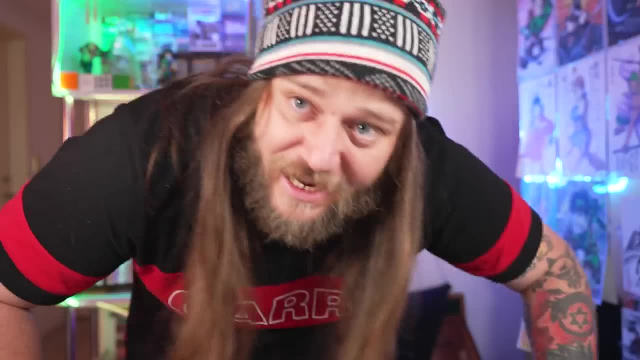 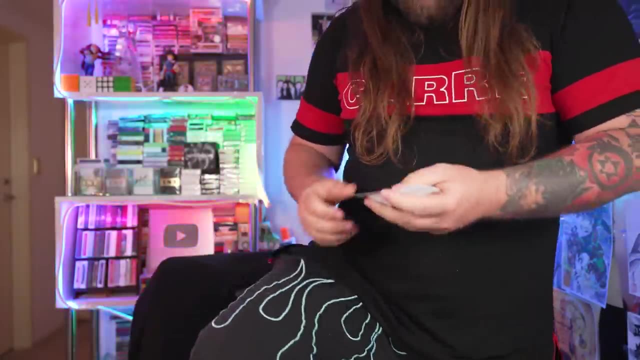 looks like that card disappears completely. and i know what a lot of you are thinking. you're thinking: do i need a table to do that? no, you don't check it out, man. one perfectly good knee will do the same thing. it'll look like that card is on the